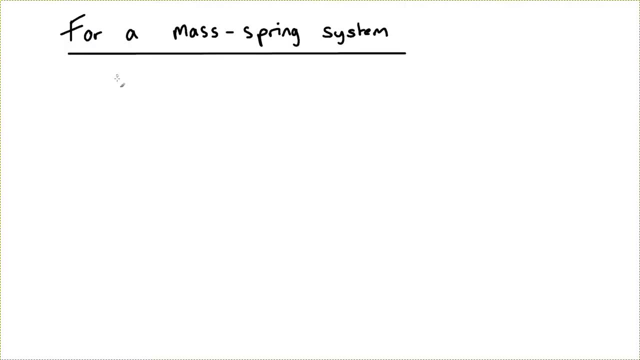 And there you go, you count the oscillations. So for a mass spring system, once we determine the period. well, we can determine the period if we know the mass and the spring constant. So the relationship there is: t equals 2 pi squared m over k, where m is the mass we've suspended on the end. 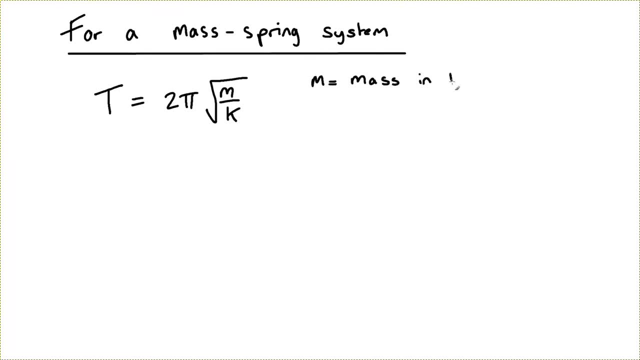 of our spring in kilograms, and k is the spring constant, or sometimes call it the force constant of the spring, which will be measured in newtons per metre, And that can easily be determined if we get the force needed to cause a certain extension in the spring, and then just f equals k. 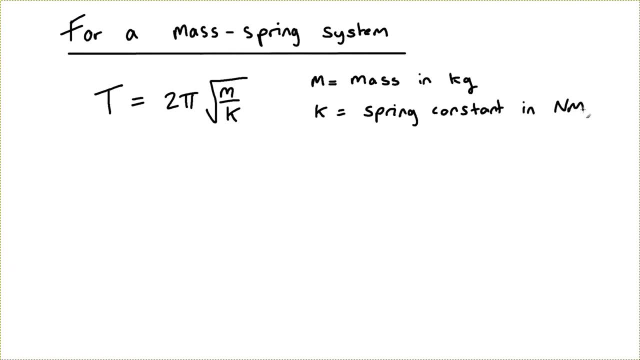 delta l. f is the force, delta l is the extension, k is the spring constant. so that's very easily determined. Of course we can plot a graph. So basically, let's say we've measured the period for different masses on the end of the spring. If we plot a graph of period in seconds against, 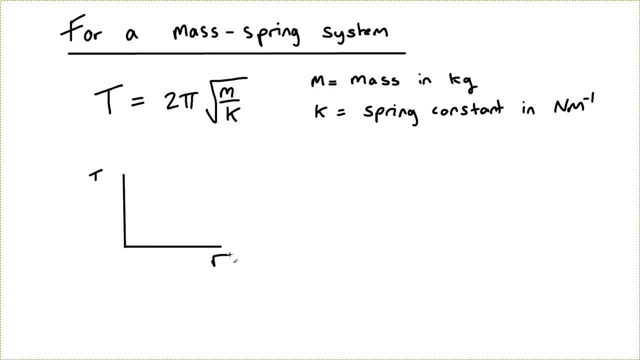 square root of the mass in kilograms. what we will get is the mass that we just measured, So that's the square root of the mass in kilograms. What we will get is the mass of k in kilograms, a straight line graph that will pass through the origin. 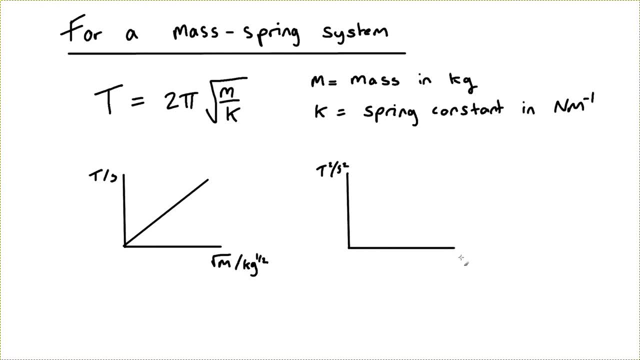 Alternatively, if we square both sides of the formula, we could plot t squared against m. And again, if we have a constant gradient, the graph would be a straight line that would pass through the origin. It's important we understand what the gradient of these graphs is going to represent. 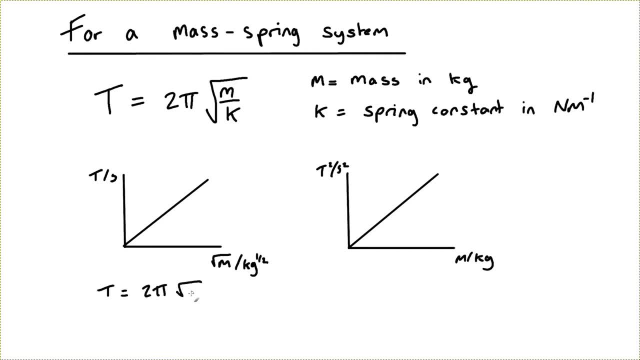 So if we compare the equation to the general equation of a straight line graph, which is: y equals mx plus c, we can rewrite: t equals 2 pi square root of m over k as 2 pi over the square root of k times the square root of m. 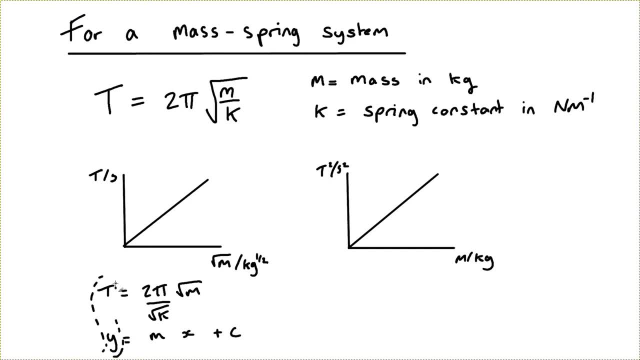 And if we do it in that form, it's very easy to see that if we plot t on the vertical y axis and we plot the square root of the mass on the horizontal axis as our x variable, then the gradient is just going to be, of course, whatever is multiplying our x variable. 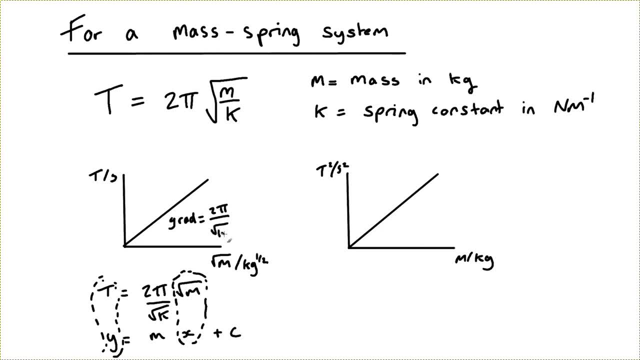 So in this case it will be 2 pi over the square root of k. If we plot the graph as t squared against m, again we can write the formula in the form: y equals mx plus c, and if we do that we can very easily see that in this time. 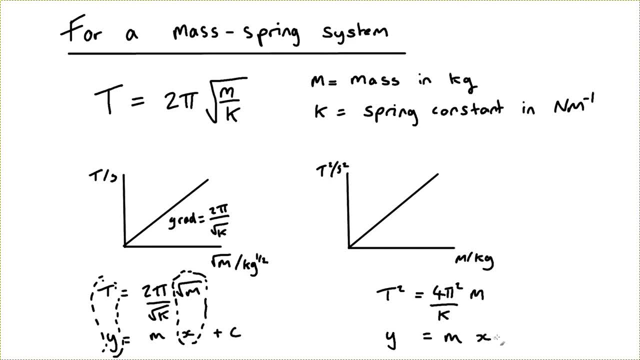 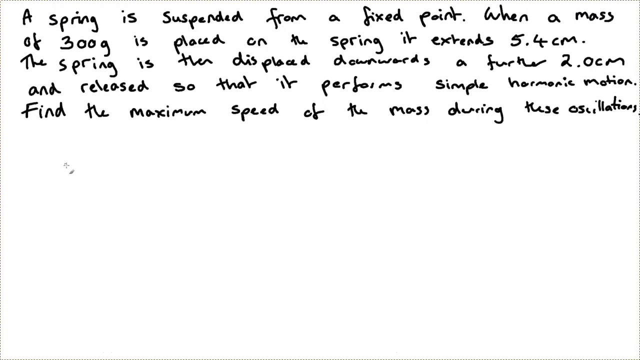 in this case the gradient will be 4 pi squared over k. So if you work out the gradient you can easily determine the spring constant from the gradient of that graph. OK, so let's sort of look at an example question involving the mass spring system. 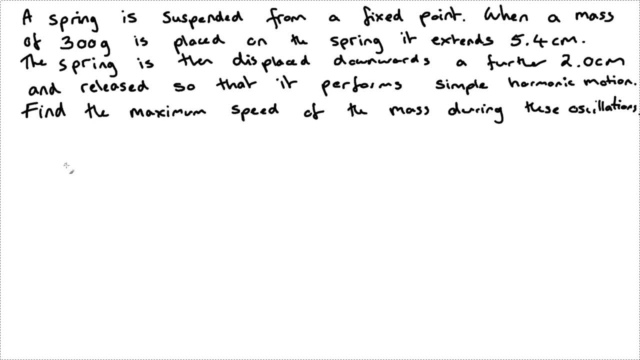 So here, let's suppose we've got a spring suspended from a fixed point similar to what we've just seen. We put a 300 gram mass on the end of the spring, and when we do that the spring extends 5.4. 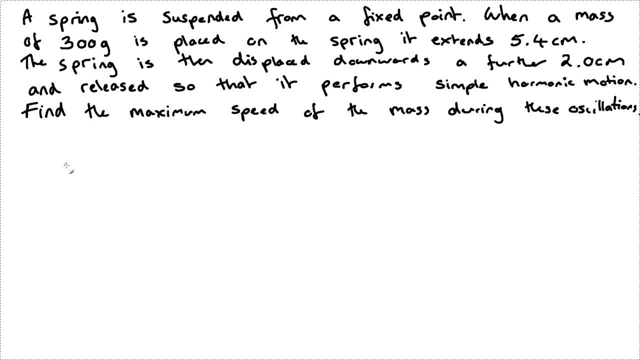 centimeters down to its equilibrium position. We then give the spring a further displacement of 2 centimeters and release it. It performs simple, harmonic motion. Can we find the maximum? Can we find the maximum speed of the mass during those oscillations? 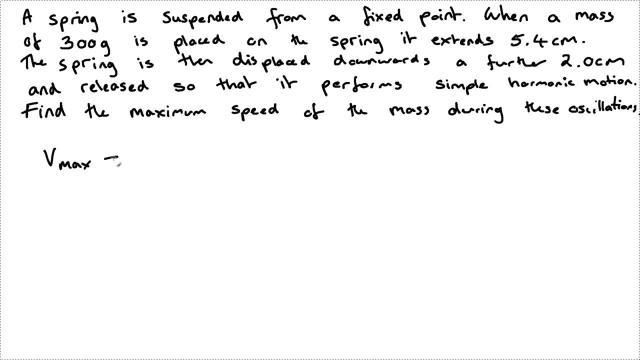 Well, we know a formula for maximum speed of simple harmonic motion and that is that v max is 2 pi f a. So if we multiply 2 pi, the frequency is 1 over period by the amplitude. so we're extending it 2 centimeters 2 times 10 to the minus 2 over meter we could determine v max. 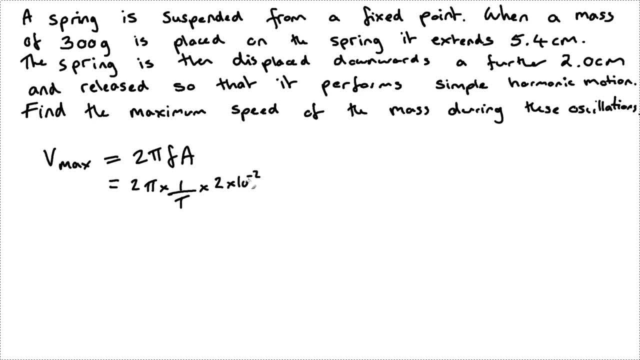 The problem is we don't know the period at the moment, but of course for a mass spring system we can work out the period Using. t equals 2 pi square root m over k. So if I know, I've got a mass of 0.3 kilograms. ah, of course we don't know the spring constant. 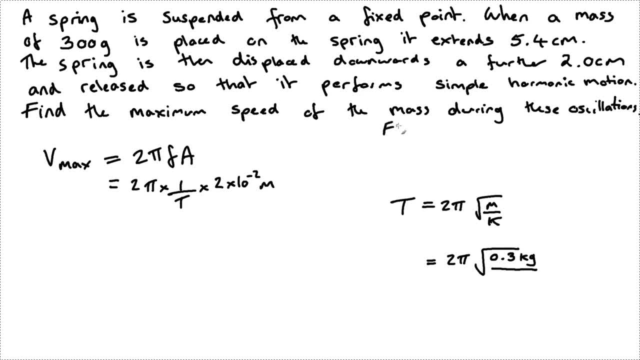 But we do know that, initially, when we put 300 grams on the end of the spring, it extended 5.4 centimeters to reach an equilibrium position where the weight pulling the spring downwards was matched by the tension in the spring. So what we can do then is use the formula f equals k. 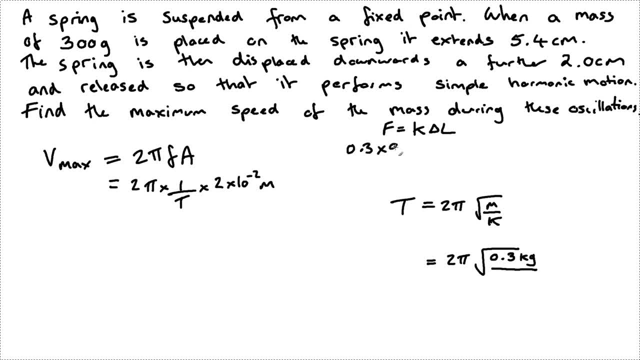 delta L Hooke's law, basically, and if we do that, we can put the weight of the mass in as the force that's causing the spring to extend. We know that that weight extends the spring by 5.4 centimetres, or 5.4 times 10, to the minus 2 of a metre, and it is then simply: 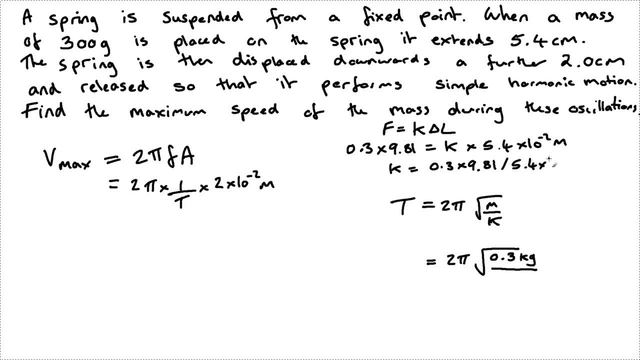 a case of rearranging the formula to work out the spring constant. Now, of course, once we've worked out the spring constant, all we need to do then is to place that in the formula, So we can put that into our formula. so T now equals 2 pi square root. 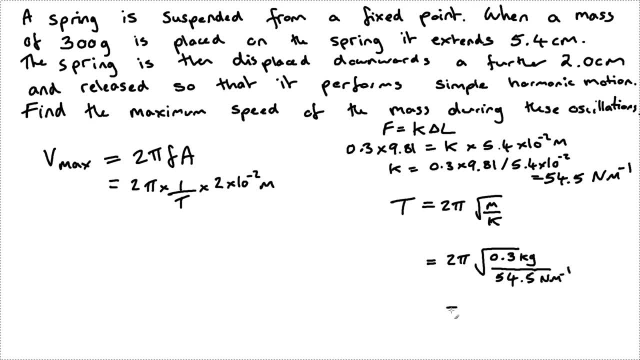 0.3 over 54.5 Newton per metre, our spring constant, and if you put that in your calculator, you can work out the period, which will come to be 0.466 seconds. Now, of course, once we've got that period, we know the period of the oscillations, we can work out the frequency. 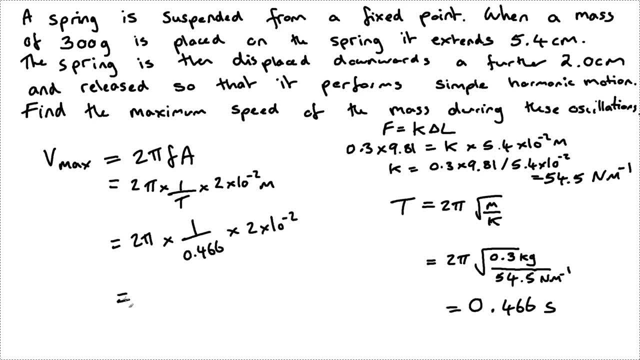 we already know the amplitude. we're giving the spring a further displacement of 2 times 10 to the minus 2 metre to set it into oscillations, and therefore we can determine Vmax 2 pi times 1 over 0.4.. 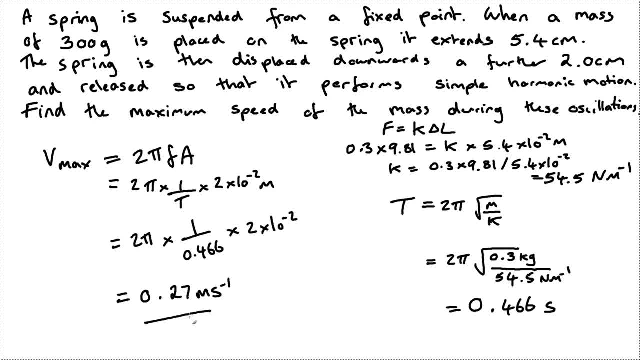 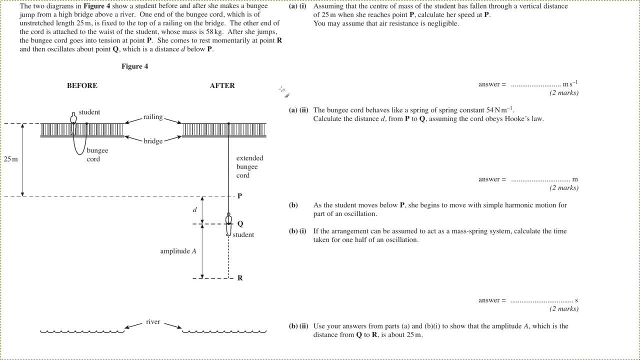 Vmax 2 pi times 1 over 0.466 times 2 times 10 to the minus 2 will equal 0.27 metres per second. and there we go. Okay, we've got another question here which refers to a bungee jump. So it says the two. 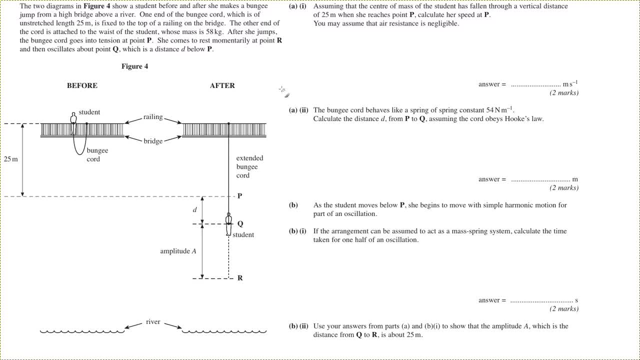 diagrams in figure 4 show the student before and after making a bungee jump. So she jumps off the bridge on the end of this bungee cord and it says here: the bungee cord has got an unstretched length of 25 metres. 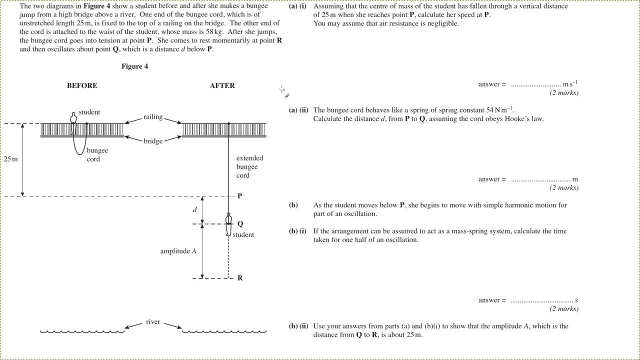 It's fixed to the top of the railing and the other end is attached to her waist. She's 58 kilograms. She jumps off the bungee cord. The bungee cord will go into tension at point P and she will then come to rest momentarily at point R and will then oscillate about point. 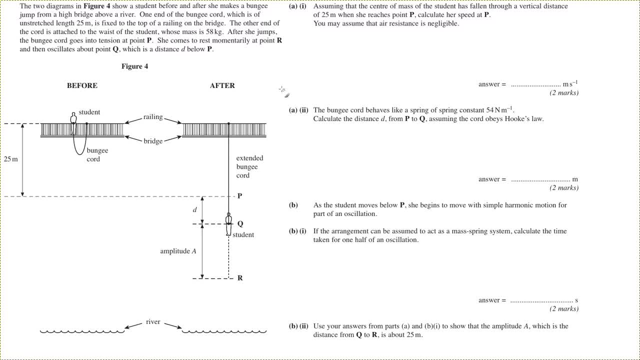 Q: Okay, so let's just think about that Basically. at point P the bungee rope is going to go under tension. Obviously she's been falling off the bridge so she'll have a speed at that point. So she'll be travelling down quite quickly, Basically, as the bungee rope stretches. 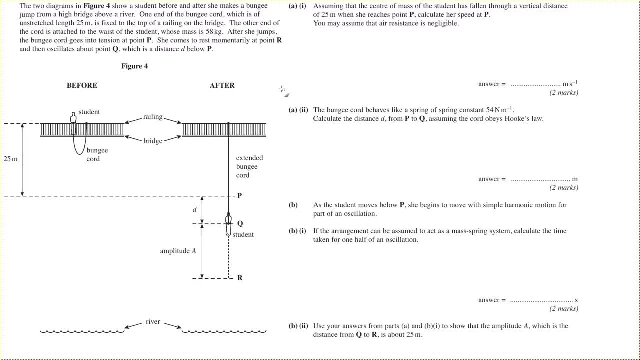 we're going to have a conversion of gravitational potential energy and kinetic energy into elastic potential energy. as she drops, Point Q is going to be the centre point of the oscillation. What she will do then is further extend the bungee into point R. Q to R will be the amplitude. 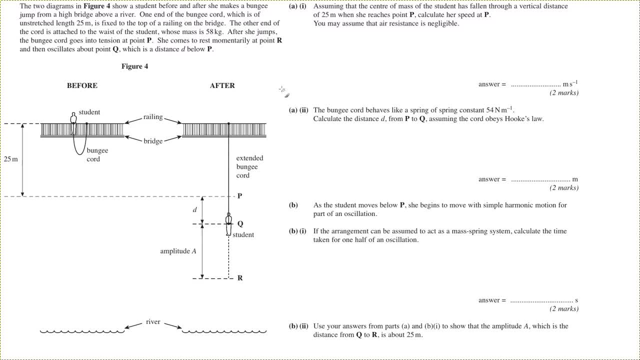 of her oscillation and then she'll oscillate and come back up again and rise just somewhere above point P. Assuming that the centre of mass of the student has fallen through a vertical distance of 25 metres when she reaches point P, calculate her speed at P. You may assume that air resistance 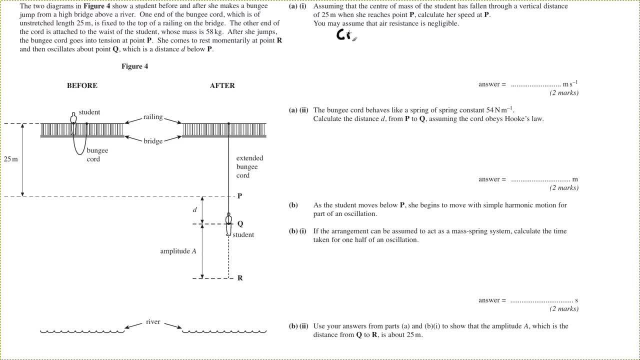 is negligible. So that's going to be a fairly straightforward question. really, It's just conservation of energy. She's been falling from the bridge, she's been losing gravitational potential energy and she's been gaining kinetic energy. We know GPE is Mg, delta A. 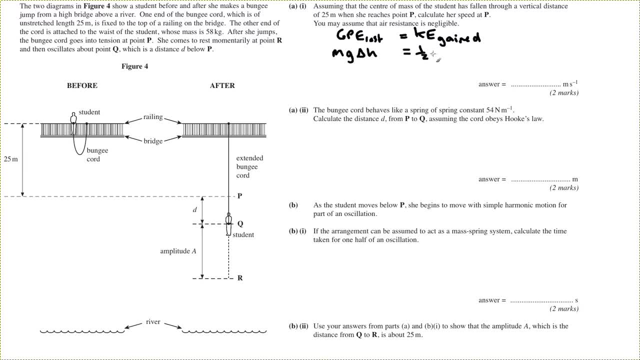 H at the Earth's surface, Kinetic energy is half mv squared. We can equate those two. Of course the mass will just cancel out. We can put in the values, Cancel the mass, Rearrange the formula and we will work out her speed at point P. 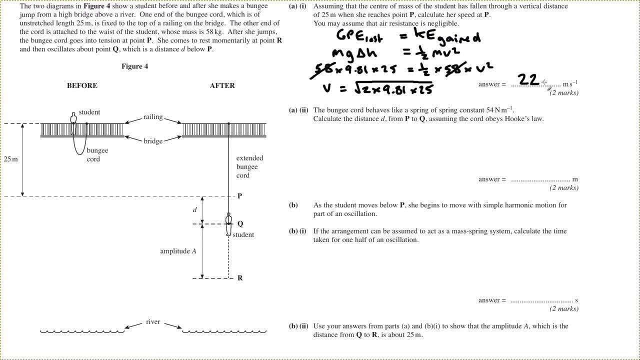 And that comes to 22.1 metres per second. The bungee cord behaves like a spring of spring, constant 54 Newton per metre. Calculate the distance D from P to Q, assuming the cord obeys Hooke's law. What we know is that Q is the. 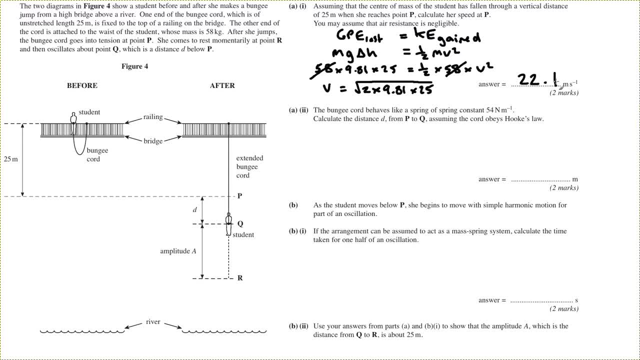 point at which she oscillates about. It's the centre of her oscillation. Therefore, at point Q the forces are going to be balanced. The tension in the bungee cord acting upwards will equal the weight acting downwards. So we can just use: F equals K, delta L. Basically we're working out the spring constant here. 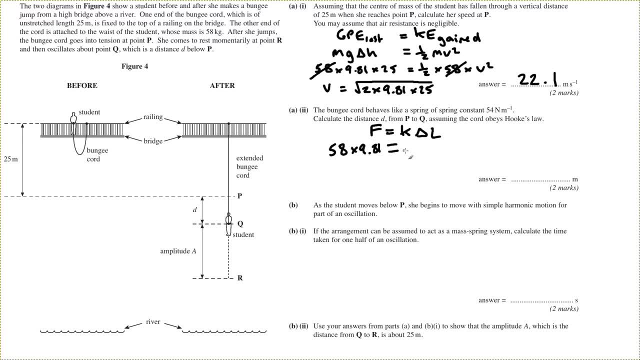 We've got the spring constant. we're working out the extension. Essentially, it's the extension in the spring that will cause the tension in the spring to equal her weight, because we're looking at the equilibrium position of the simple harmonic motion, where we know the forces are going to be balanced. 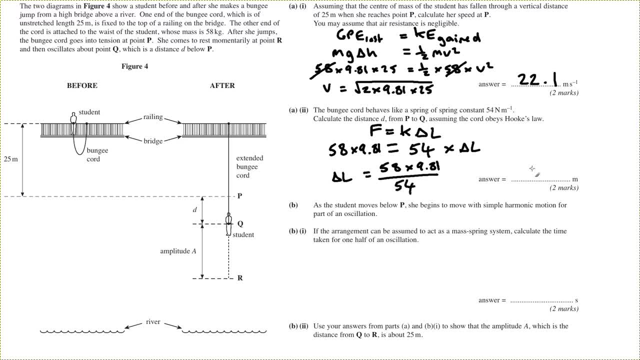 So to do that, F equals K, delta L. Put the numbers in, We can rearrange it. It comes out as 10 and a half metres. We'll round it to two significant figures, which is an appropriate number of significant figures here, And it's 11 metres. 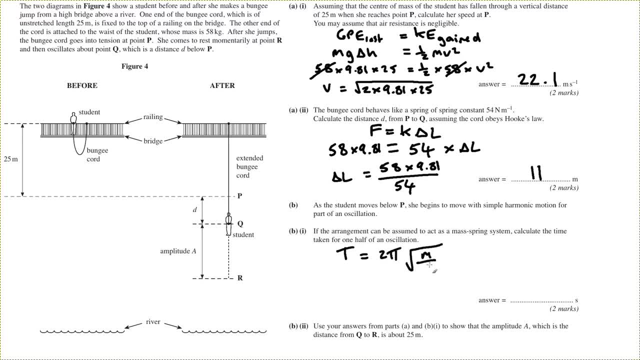 The arrangement can be assumed to act as a mass spring system. Calculate the time for one half of an oscillation. Well, we know how to calculate the time of an oscillation for a mass spring system. T equals 2 pi square root m over K. The formula is in our data. 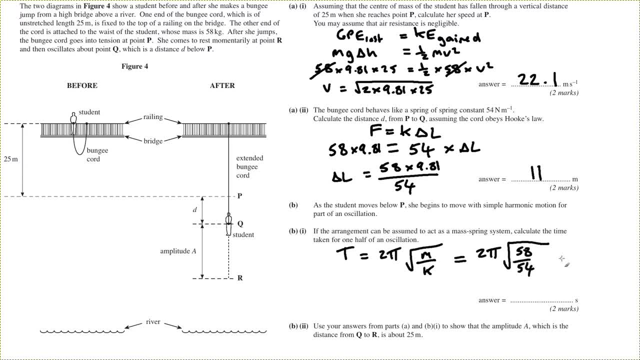 book. We know the mass, We know the spring constant. We've been given that earlier in the question. Again, it's just a case of putting the numbers in and we will work out a value for the period. And the period comes to 6.51 seconds. So if we halve that, because it's asked us for half, 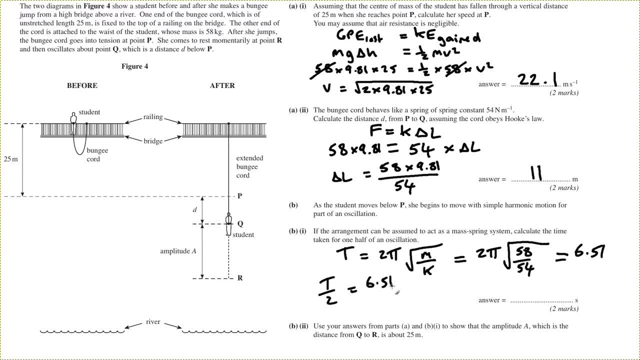 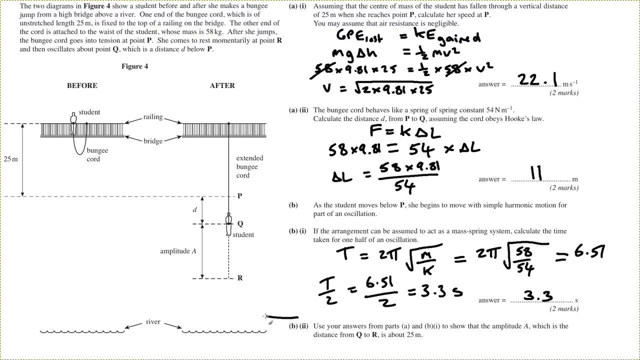 in this case the 피 is done. But what does that mean then? Well, it means the amplitude is less than�� is less than pi. So we maybe само-cons. So in first sort of quarter period they moved down from Q to R, And as they go back back up they're gonna oscillate at an equal distance. 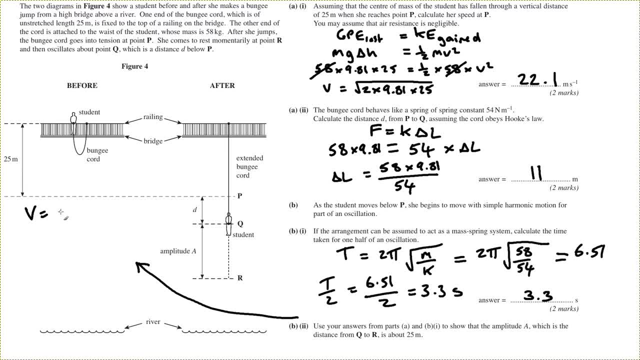 above Q, which is gonna take them back up, up above points P, And that would be one. that would be the oscillation. So what we can use here is the formula for speed at any point in the oscillation, Because we know the speed that you would have. 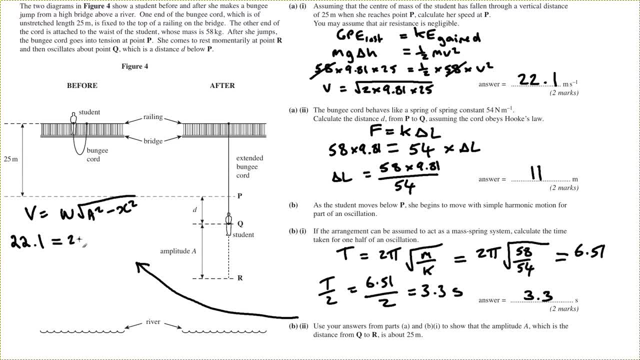 at point P. we've worked that out in a part 1. we know the displacement at point P and we know the period, so we can work out the frequency of the oscillations. so we can use that formula basically to work out the amplitude, because we know. 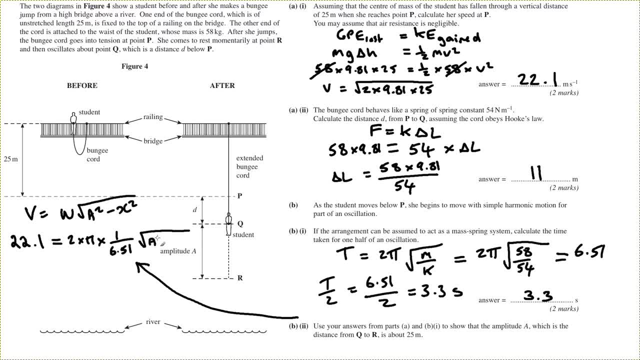 everything else. so it's just realizing that essentially P is not the end of an oscillation, it's not the top of the oscillation. she will oscillate above that. ok, P distance Q to P is less than the amplitude of the oscillation. so essentially she goes down from Q to R, she's converting while kinetic and 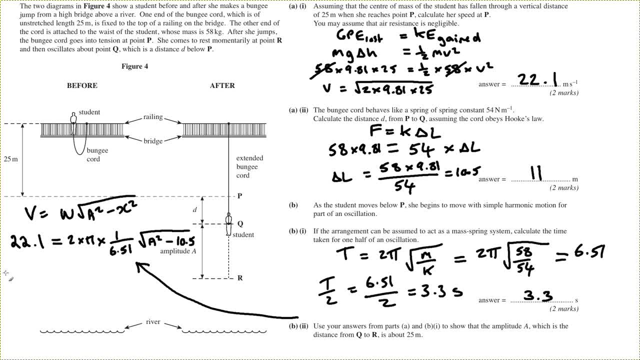 gravitational potential energy into elastic potential energy and then, as the bungee cord contracts, again pulls her back up, she's converting that elastic potential energy back into gravitational potential energy and kinetic energy at Q, but then that's all going back to gravitational potential energy as she reaches the top of her bungee jump. And there we go. So we can. 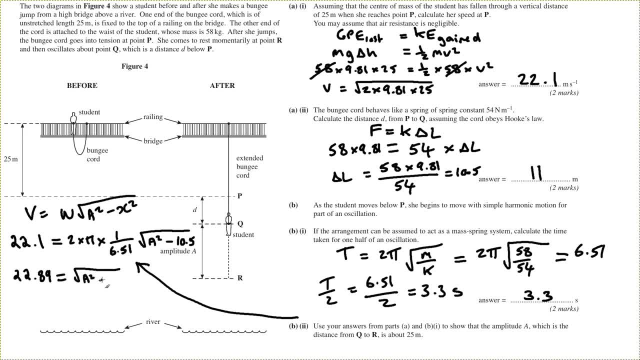 put the numbers into the equation. The question, then, is just rearranging it. So we've got 22.1 equals 2 pi over 6.51 times the square root of a squared minus 10.5.. That should be 10.5 squared there. Just add that in And then it's the case of just rearranging. 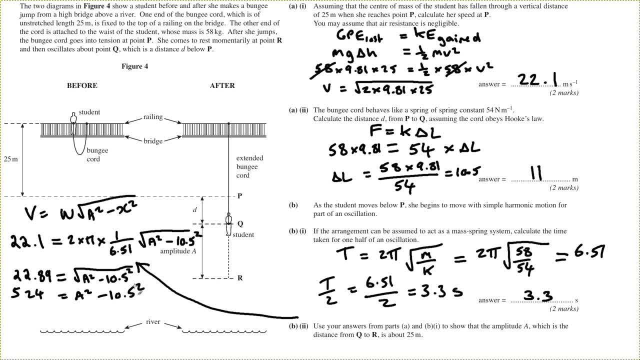 that equation. So we can times 3 by 6.51, divide by 2 pi, square both sides, We come out with 524 equals a squared minus 10.5 squared. So then a squared is going to be the square root of 525 plus 10.5 squared. So there we go. 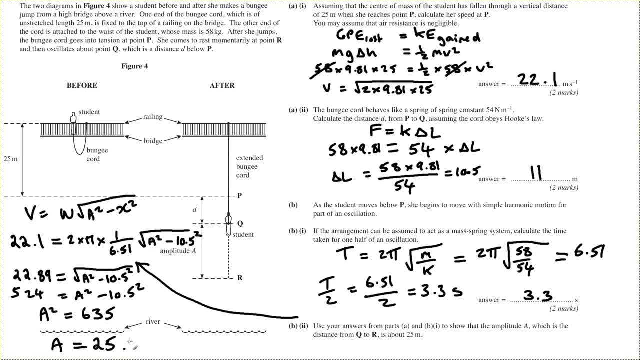 We'll work that out And we come to 25.2 metres. So just to make that clear, as the student dropped from point Q went down to point R- that's the amplitude of the oscillation- And then what they would have done is they would have oscillated on the way back up. come back.